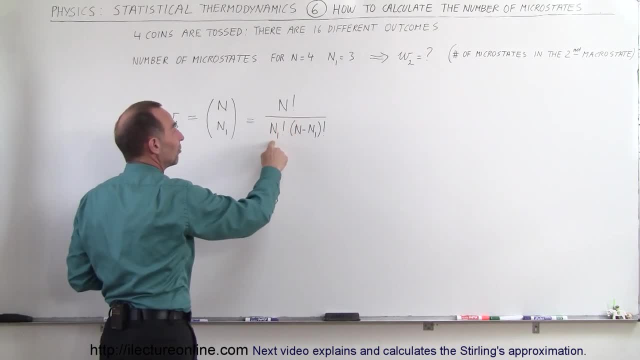 And so the equation becomes n factorial divided by n sub 1 factorial, times n minus n sub 1 factorial. So this is the total number of entities factorial. this is the number of entities that have heads, and this would be the number of entities that have tails out of the total of four. 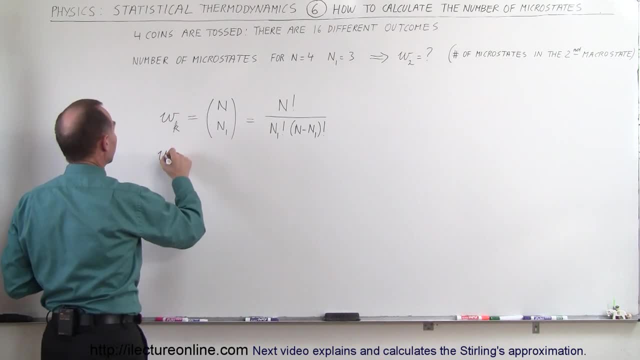 So in this case, since we're looking for W sub 2, that would be equal to there's four coins, and in that microstate there are three coins that have heads. So this would then become 4 factorial divided by 3 factorial times 4 minus. 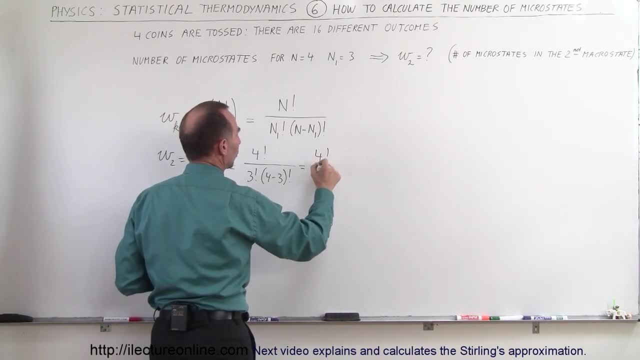 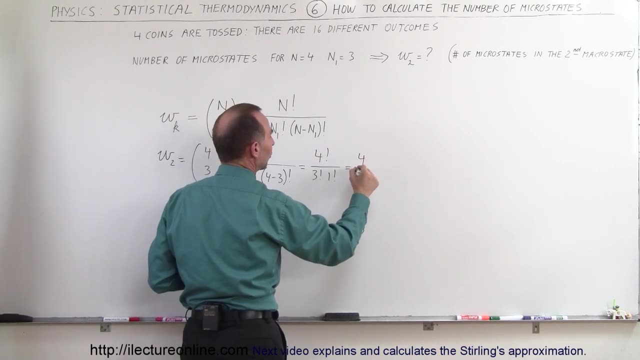 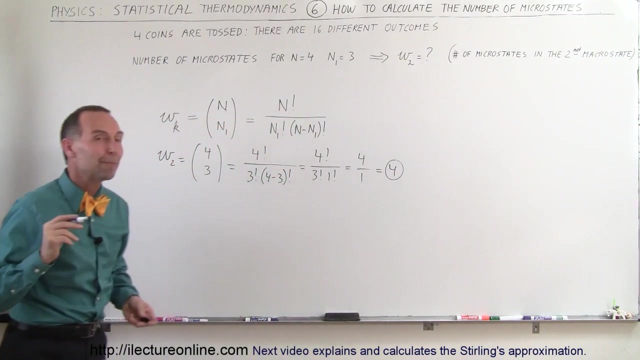 3 factorial, which is equal to 4 factorial divided by 3 factorial times 1 factorial, And so 4 factorial divided by 3 factorial is simply 4, and, of course, 1 factorial is simply 1, so it's 4 divided by 1, or 4, which means that particular microstate has four microstates. 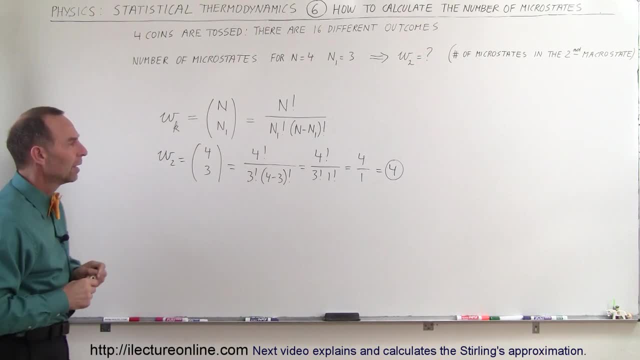 That makes it kind of nice. That's pretty a pretty good equation. Can we use that equation for larger numbers? And of course we can use it for larger numbers. That's why we have the equation for something as simple as this. Subtitles by the Amaraorg community. 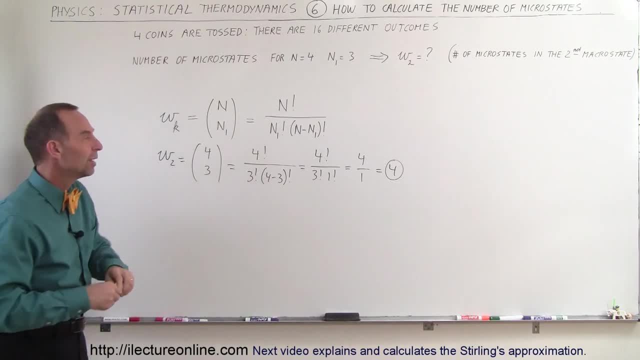 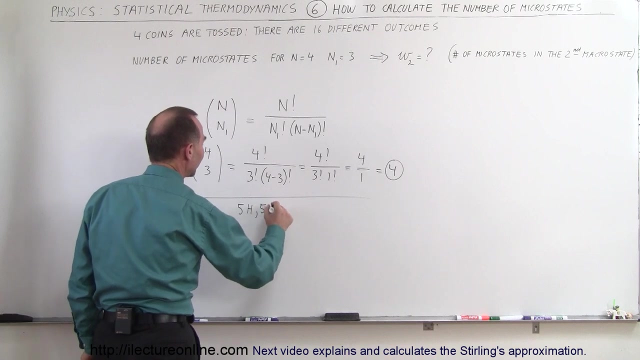 We probably don't even have to use that equation, but what if we have the situation as follows: What if we have 10 entities? We're going to throw 10 coins and I want to know the number of microstates in the microstate where I have 5 heads and 5 tails. 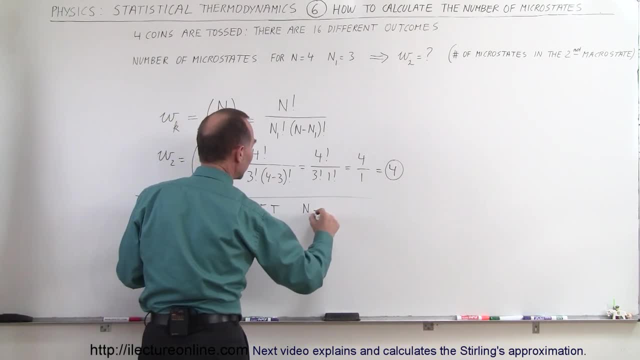 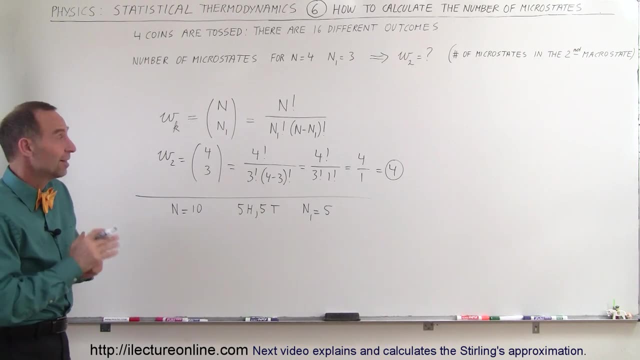 In other words, since n is equal to 10,, that means n sub 1 is going to be equal to 5.. Now how many microstates, or how many microstates are there in that particular microstate? Now, without this equation, 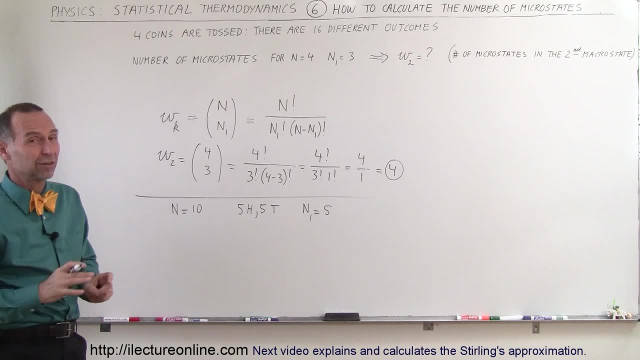 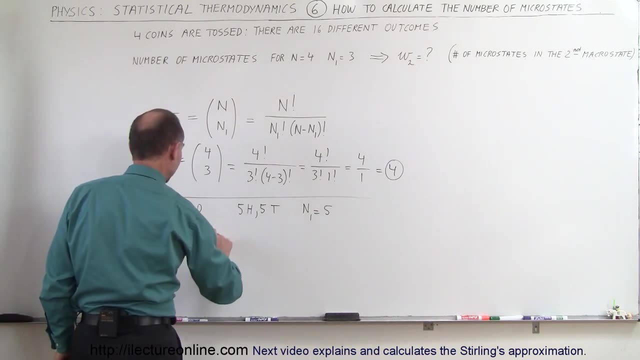 You'll be sitting there for a long time with a pen and a piece of paper trying to figure it out. But this equation makes it nice. So we're going to find omega, which is equal to 10,, 5,, which is equal to 10- factorial. 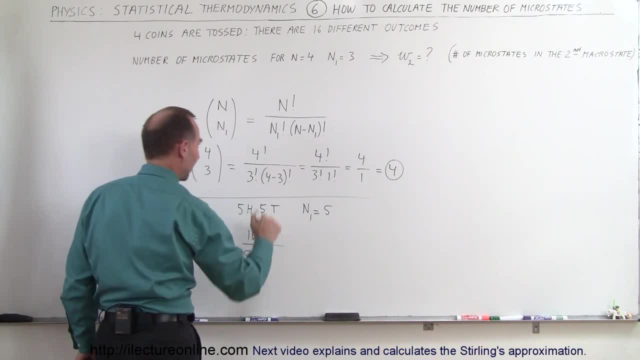 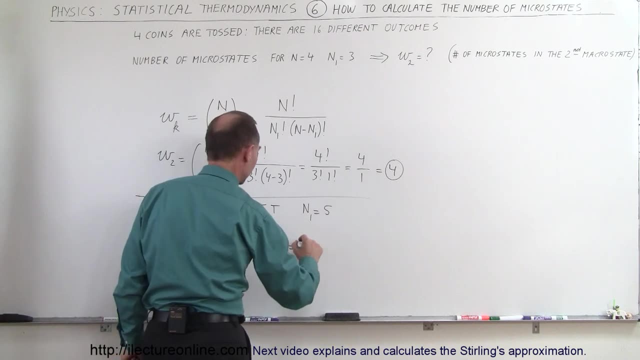 divided by 5 factorial and of course, 10 minus 5, that would also be 5 factorial. In that case, 10 factorial divided by 5 factorial is equal to 10 times 9 times 8 times 7 times 6,. 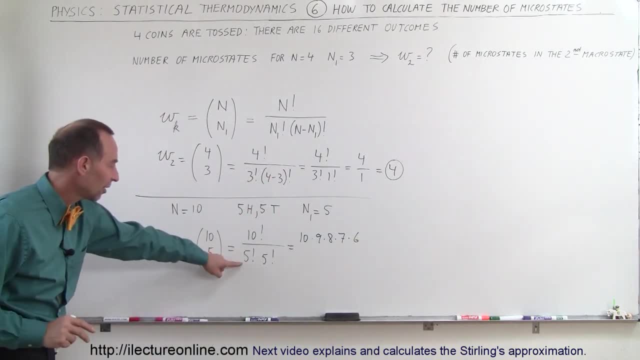 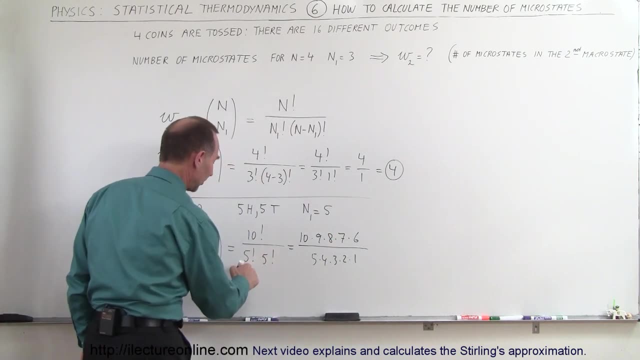 because 5, 4, 3, 2, 1 multiplied together is cancelled out by one of these. and then we have to divide that by 5 times 4 times 3 times 2 times 1.. So this cancels out the 5 times 4 times 3 times 2 times 1 out of the numerator. 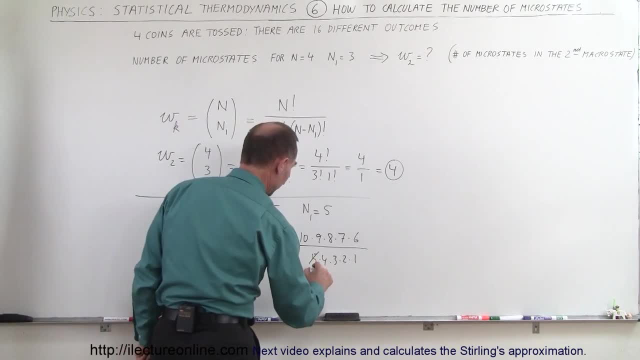 Okay, now we can simplify things a little bit more. So this 5 becomes a 1.. When we divide that by 5, it becomes a 2.. This 2 goes to 1.. This goes to 1.. We have a 9 and a 3, so 3 goes into 9 three times. 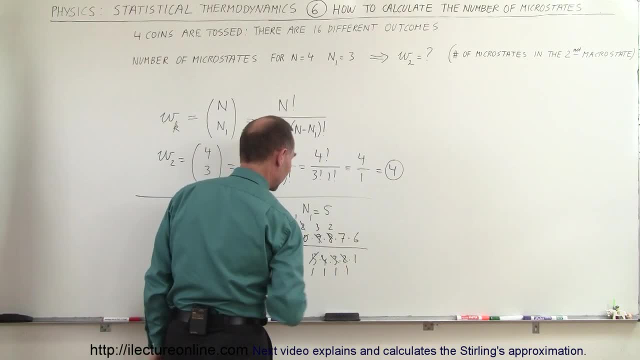 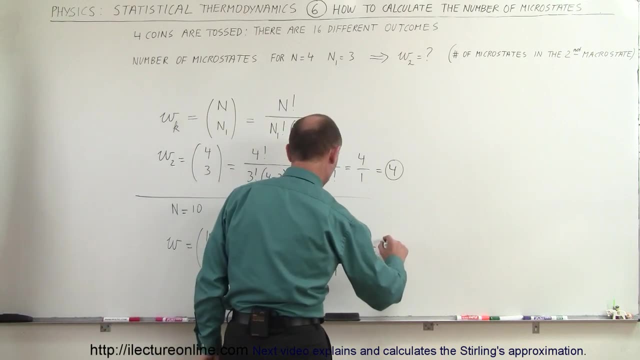 and 4 goes. 4 goes into 8, two times like that, And so now we have 1s in the denominator. Now I simply have to multiply the numerator numbers that I have left, So this would be equal to 3 times 2 times 7 times 6.. 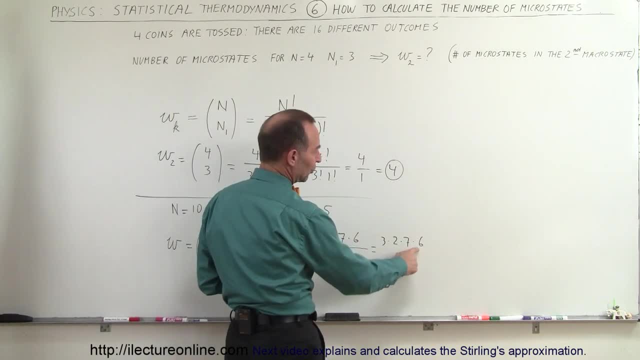 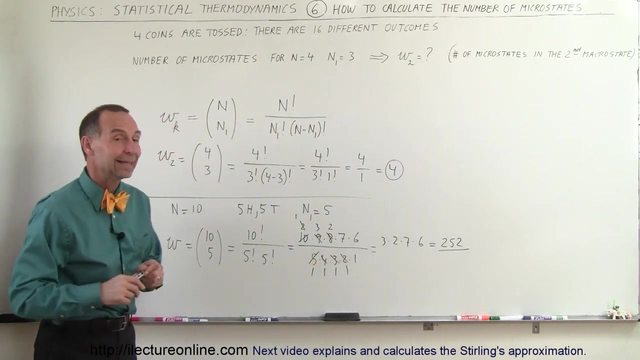 All right, 7 times 6 is 42, times 2,, that would be 84, times 3,, that would be 84,, that would be 252.. Okay, that means that in the case of flipping 10 coins, 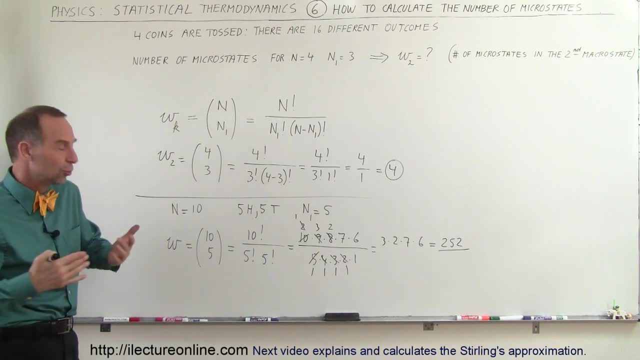 and any of them can be heads or tails. so there's two energy states, so to speak, or two states, and we want to find out how many different ways in which coins can land when you have 10 coins, so that 5 of them will be heads and 5 of them will be tails. 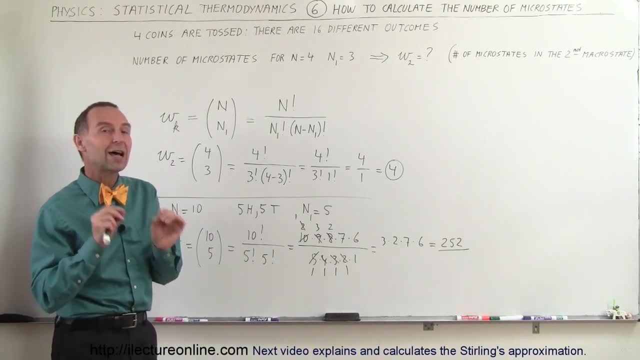 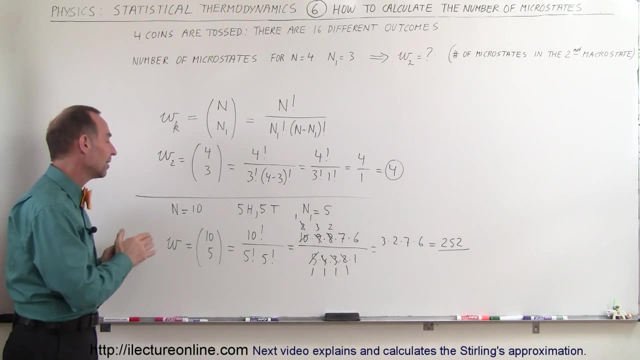 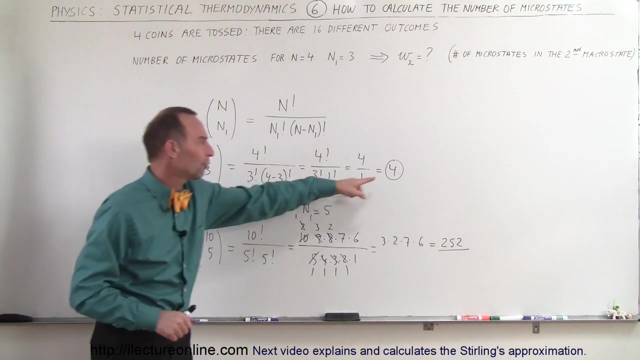 there are 252 combinations, 250 outcomes like that, which means there are 252 microstates in that particular microstate, that represents 5 heads and 5 tails. Wow, that's a huge number compared to the number 4 when we only toss 4 coins. 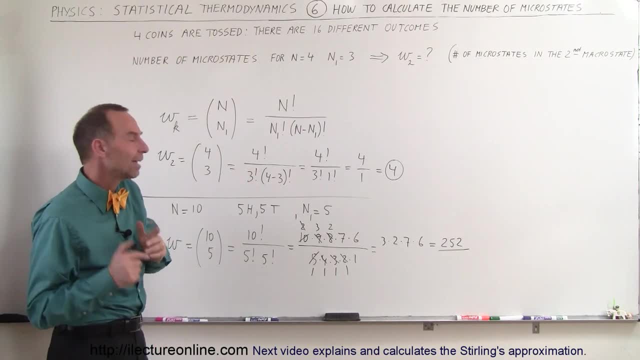 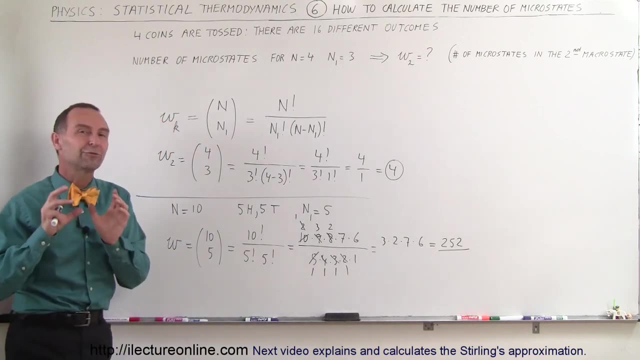 when we have 3 heads and 1 tail and, of course, in the case where we have 2 heads and 2 tails, the number would be 6 outcomes, but here it's grown to 252.. Just by going from 4 coins to 10 coins. 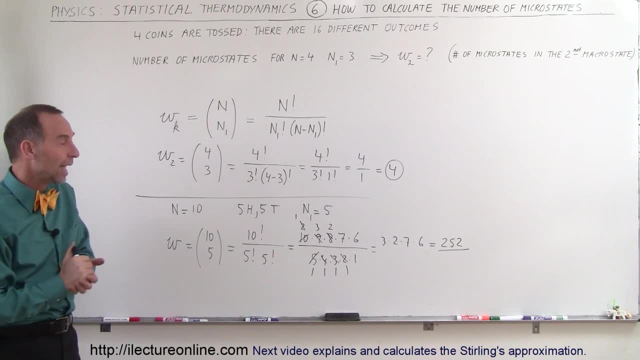 the numbers are getting quite large already. Now imagine what's going to happen when we go from 10 coins to 100 coins, from 100 coins to 1,000 coins, or from 1,000 coins to to Avogadro's number, 10 to the 23.. 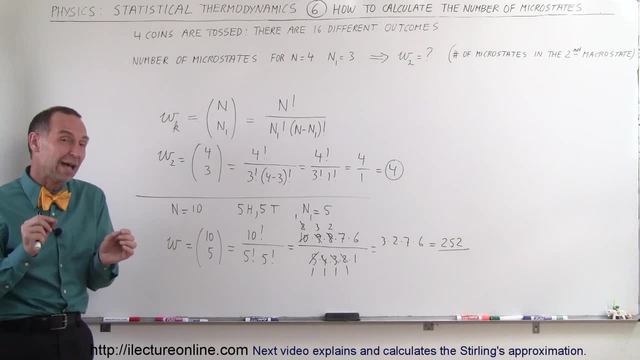 Well, 6.02 times 10, to the 23,, of course. So imagine the enormous quantity of numbers, the quantity of entities we'd have in those particular cases. You can imagine that these numbers become astronomical. That's why trying to calculate them one by one doesn't make a lot of sense.